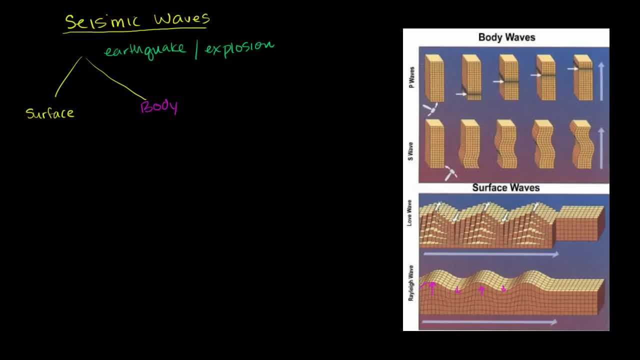 The love waves are essentially the ground shifting left and right. So here it's not moving up and down, but here it's moving. If you're facing the direction of the wave movement, it's moving to the left here. Here it's moving to the right. 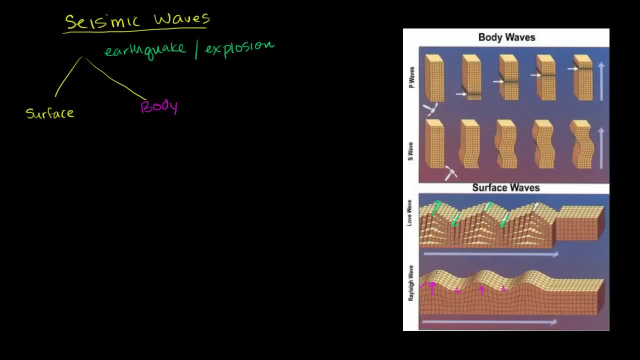 Here it's moving to the left, Here it's moving to the right. In both cases the movement of the surface wave is perpendicular to the direction of motion, So we sometimes call these transverse waves, And these are essentially analogous to, as I said, kind of what we see in water waves. 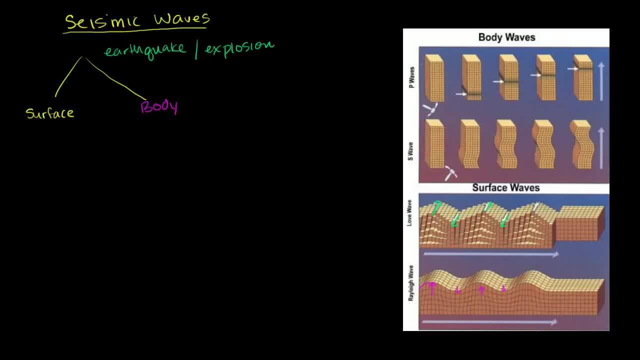 Now, the more interesting thing are the body waves. Because the body waves, first of all, they're the fastest moving waves And these are also the waves that are used to figure out the structure of the Earth. So the body waves come in two varieties. 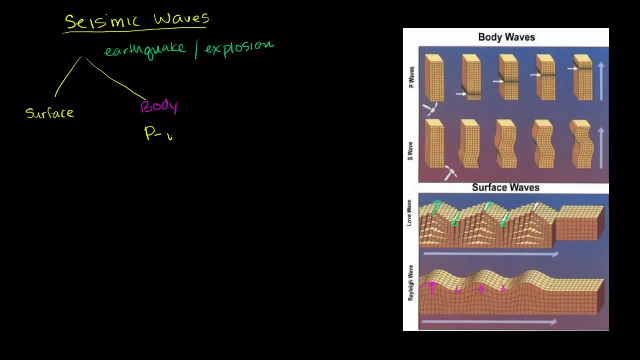 You have your P waves or primary waves. You have your P waves and you have your S waves or secondary waves, And they're depicted right over here, And this is actually energy that's being transferred through a body, So it's not just moving along the surface of one. 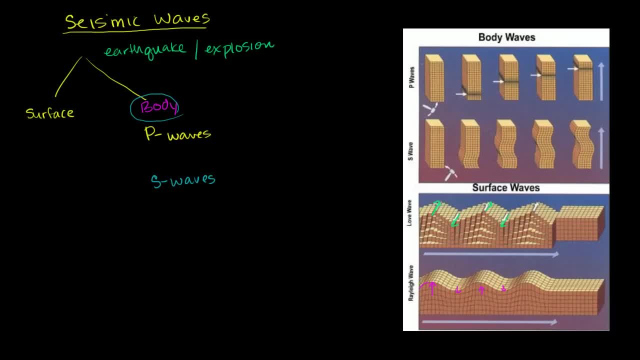 And so here in this diagram that I got from Wikipedia, which I think Wikipedia got from the US Geological Survey, we have a hammer being hit on some rock or whatever, And what you see is right when the hammer gets hit at this end of the rock. 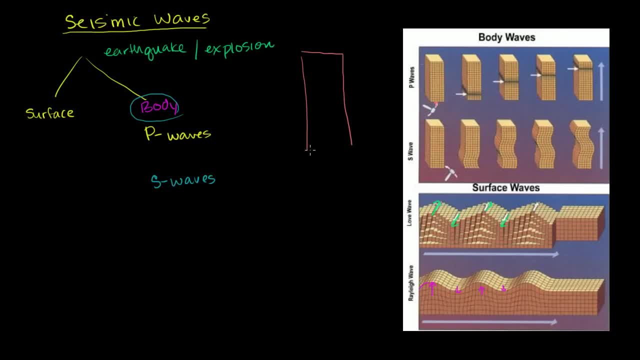 and I can zoom in a little bit. So let's say, I have this rock over here And I hit it right here, And I hit it right over here with a hammer or something. What that's immediately going to do is it's going to compress the rock. 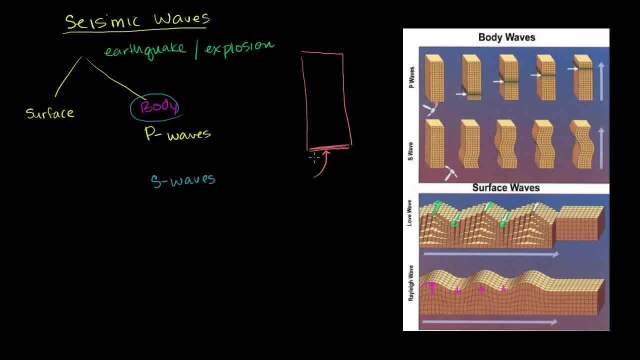 that the hammer comes in touch with. It's going to compress that rock, But then that energy- essentially the molecules- the molecules are going to bump into the adjacent molecules And then those adjacent molecules are then going to bump into the molecules right next to it. 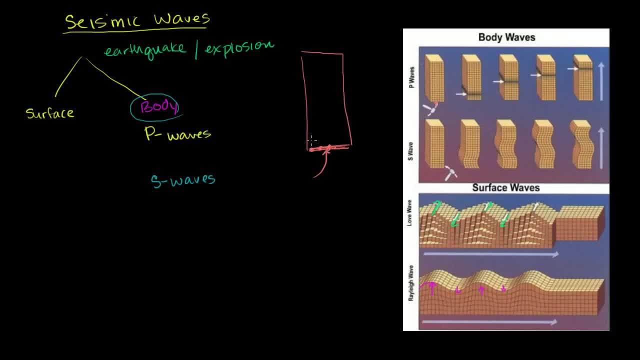 And then they're going to bump into the molecules right next to it. So you're going to have this kind of compressed part of rock moving through the wave. So these are compressed And those molecules are going to bump into the rock. These are the adjacent molecules. 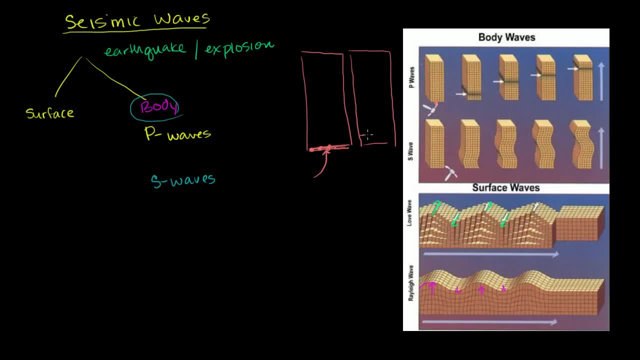 So kind of immediately after that the rock will be denser right over here. The first things that were bumped, those will essentially bump into the ones right above them, And then they will kind of move back to where they were, And so now the compression will have moved. 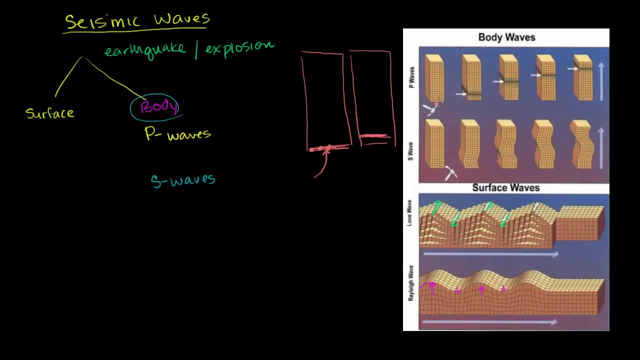 And if you fast forward it will have moved a little bit forward. So you essentially have this compression wave, You hit the hammer here And you essentially have a changing density that is moving in the same direction of the wave. In this situation, 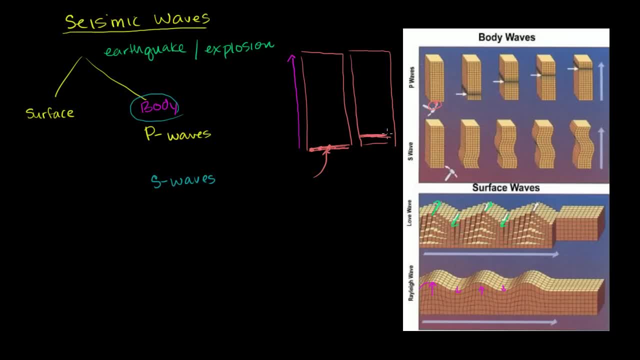 that is the direction of the wave, And you see that the molecules are kind of going back and forth along that same axis. They're going along the same direction as the wave. So those are P waves, And P waves can travel through air. 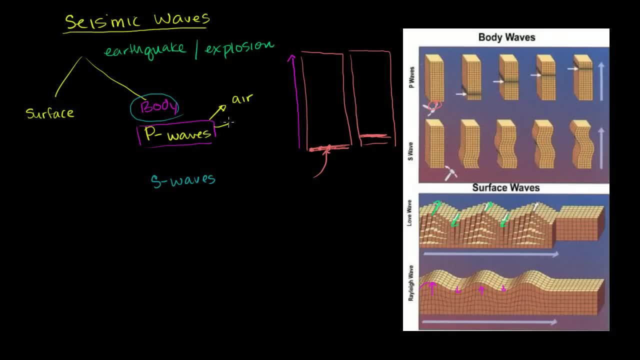 That's what essentially sound waves are: compression waves. They can travel through liquid. They can travel through liquid And they can obviously travel through solids And, depending on the air, they'll travel the slowest. They'll essentially move at the speed of sound, 330 meters per second. 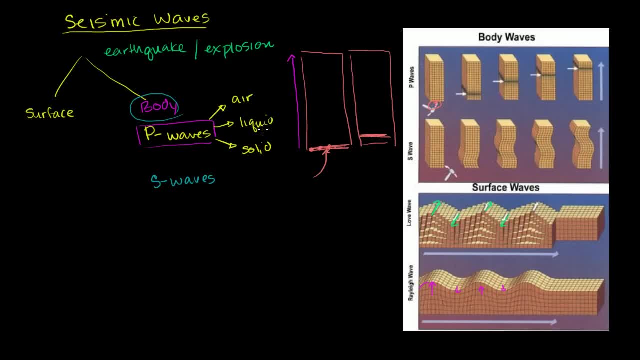 which isn't really slow by everyday human standards. In a liquid, they'll move about 1,500 meters per second, And then in granite, which is most of the kind of the crustal material of the Earth, they'll move at around 5,000 meters per second. 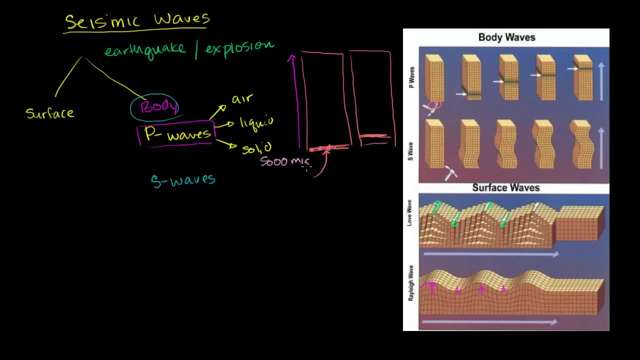 Let me write that down. So 5,000 meters per second, or essentially 5 kilometers per second. if they're moving through granite Now, S waves are essentially if you were to hit a hammer on the side of this rock. So let me draw another diagram, since this is pretty small. 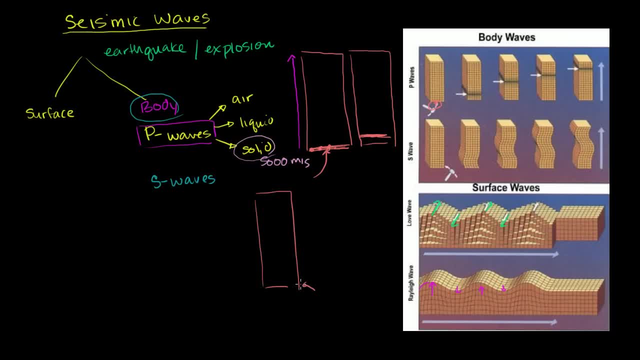 If you were to hit a hammer right over here, what it would do is it would temporarily kind of push all the rock over here. It would deform it a little bit and that would pull a little bit of the rock back with it, And then this rock that's right above it would slowly be pulled down. 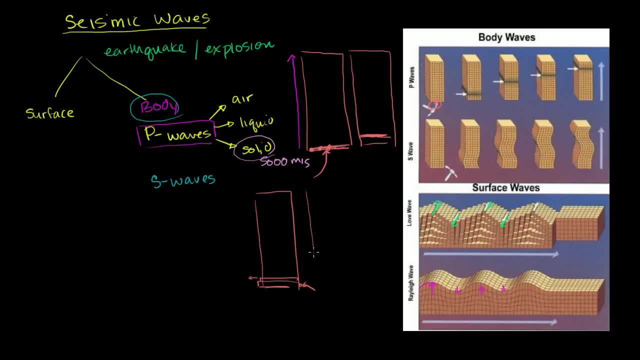 while this rock that was initially hit will be moved back up. So you fast forward, Maybe a millisecond. And now the next layer of rock right above that. maybe I should draw it. Actually, let me draw it like this: The next layer of rock right above that will be kind of deformed to the right. 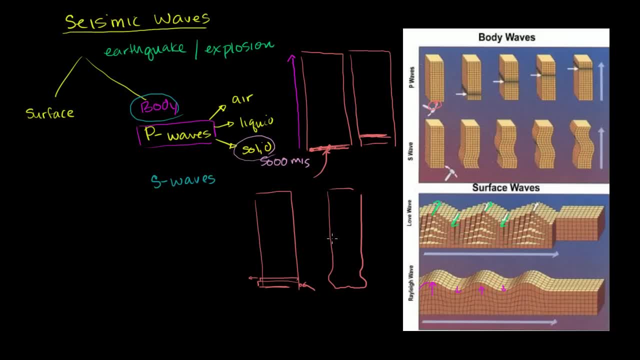 And if you keep fast forwarding it, the deformation will move upwards. And notice over here: once again, the movement of the wave is upwards, But now the movement of the material is not going along the same axis that we saw with the P waves or the compression waves. 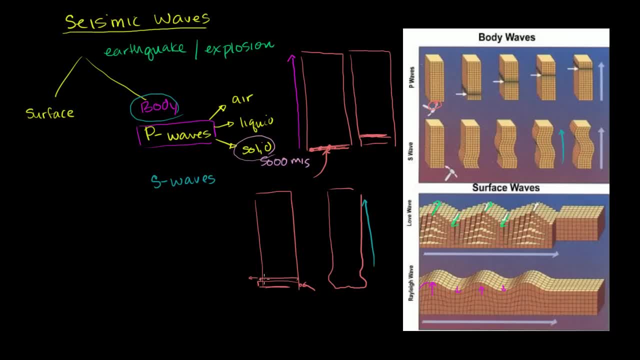 It's now moving perpendicular. It's now moving along a perpendicular axis, Or you could call this a transverse wave. The movement of the particles is now on a perpendicular axis to the actual movement of the waves, And so that's what an S wave is. 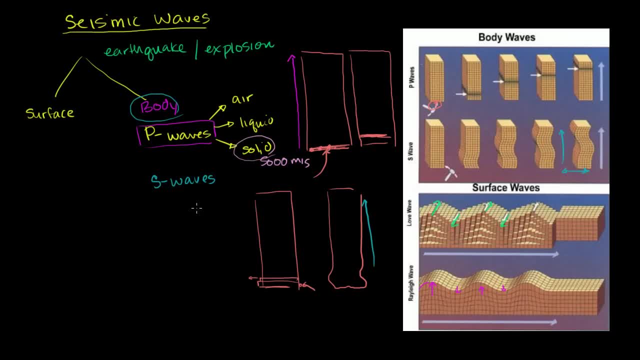 And they move a little bit slower than the P waves. So if an earthquake were to happen, you would see the P waves first, And then, at about 60% of the speed of the P waves, you would see the S waves. Now, the most important thing to think about, 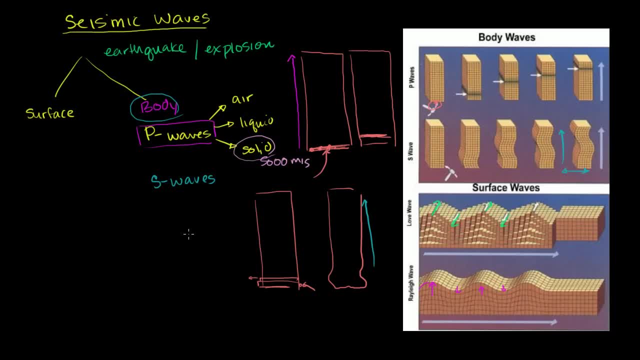 especially from the point of view of figuring out the composition of the Earth, is that the S waves can only travel through solid. And you might say, wait, I've seen transverse waves on water that look like this, But remember that is a surface wave. 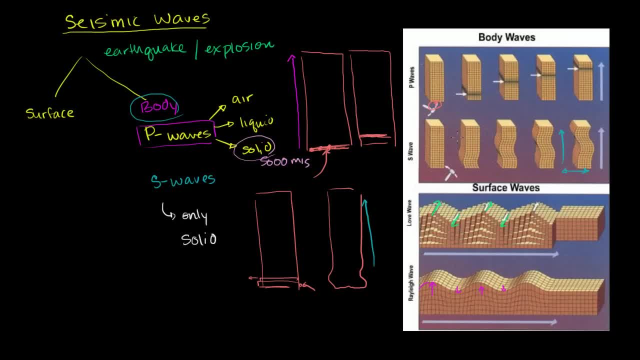 We are talking about body waves. We're talking about things that are actually going through the body of water, And one way to think about this is: if I had some water over here, Let me pull. I'll draw a cross-section of water. 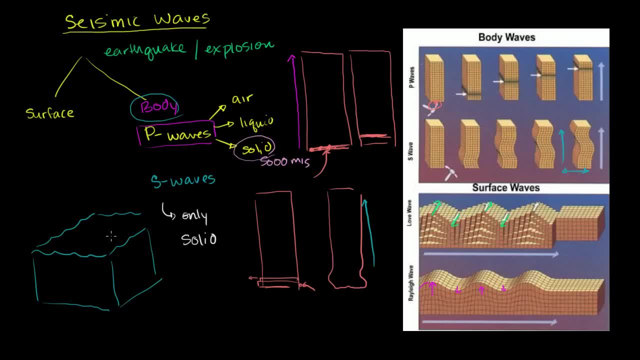 If I draw a cross-section of water, I could have drawn it better than that. Let me, If I have a cross-section of water right over here, Let's think about it And hopefully it will make intuitive sense to you If I were to compress some of the water. 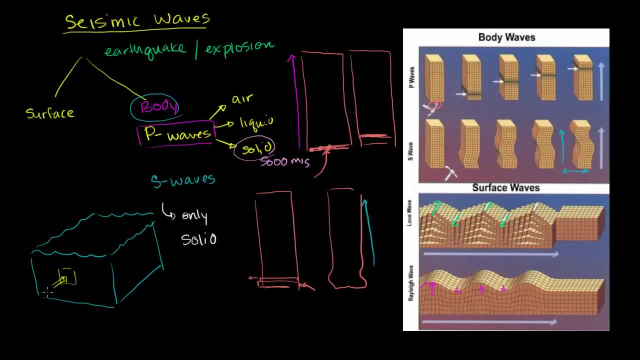 If I were to kind of slam some part of the water here with like a big, I don't know some type of, I would just compress it really fast. It would do a P wave could transmit, Because those water molecules would bump into the water molecules next to it. 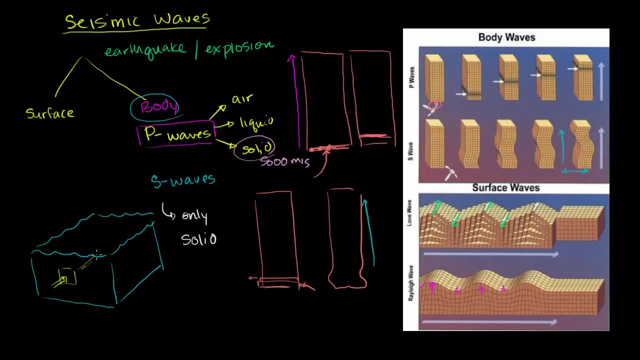 Which would bump into the water molecules next to that, And so you would have a compression wave or a P wave moving in the direction of my bump. So P waves, it makes sense, And the same thing is true with air or sound waves. 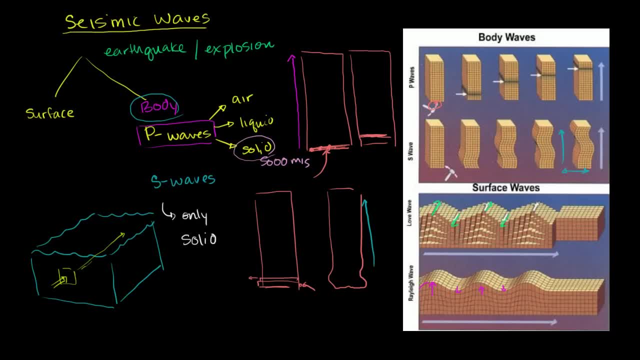 That it makes sense that it could travel through a liquid. But let's say that you, Let's say that if- And remember- we're under the water, We're not thinking about the surface, We're thinking about moving through the body of the water.